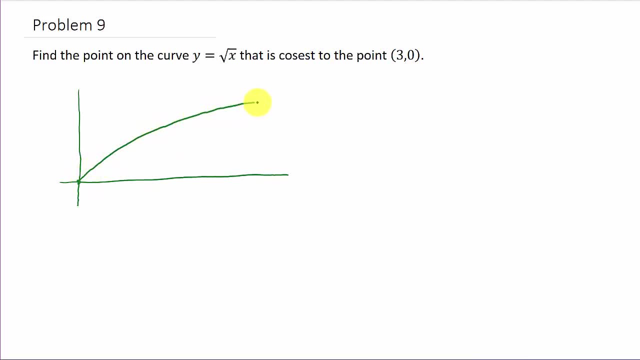 Okay, so the graph of the square root function is going to look something like this: Okay, and then we've got the point 3, 0 out here somewhere. Okay, and this is the point 3, 0.. And we want to find the distance from this point to the curve here. that's a minimum. 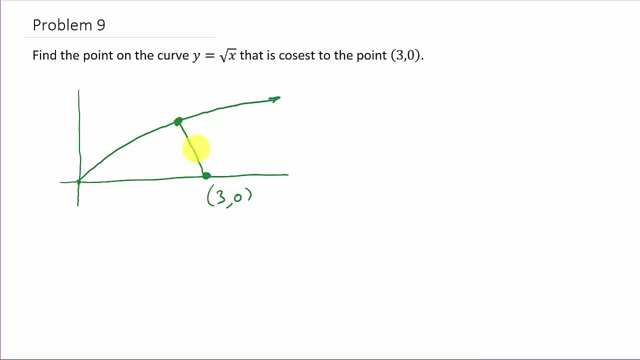 Okay now. so we're going to minimize this distance. We'll call that d, All right, so basically I'm minimizing the distance between two points. Well, do we know the distance between two points? Yeah, that's remember. the distance formula is: d equals the square root x2 minus x1, squared plus y2.. 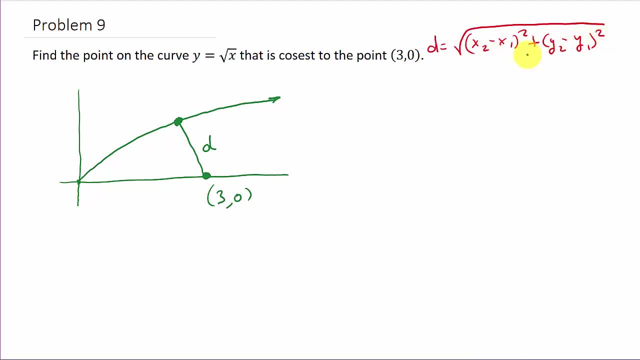 Minus y1 squared. So I need two point coordinates. All right, so we've got this point coordinate, Now I need this one. Well, if I come over one unit, if x is 1, what is y? It's the square root of 1.. 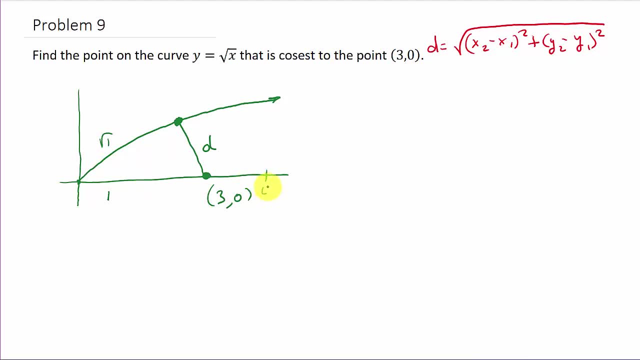 If I come over to, let's say over here to 4, what's y? It's the square root of 4.. See that If I come over x units, what's the y coordinate? It's square root of x. 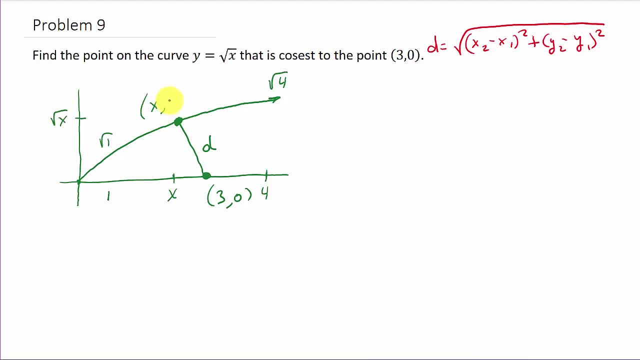 So this point here would have the coordinates x- square root of x. All right, All right, so let's look. All right, so I need to minimize the distance from the point 3, 0 to the point x- square root of x. 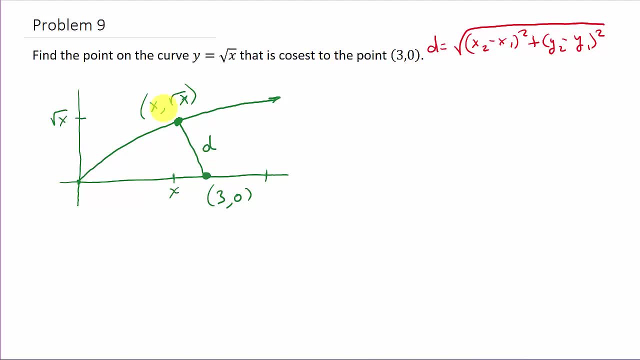 All right, so I don't know, We'll call this. we'll call this point x1, y1, and this one x2, y2.. And it doesn't matter, You could call this one x1, y1, and this one x2, y2.. 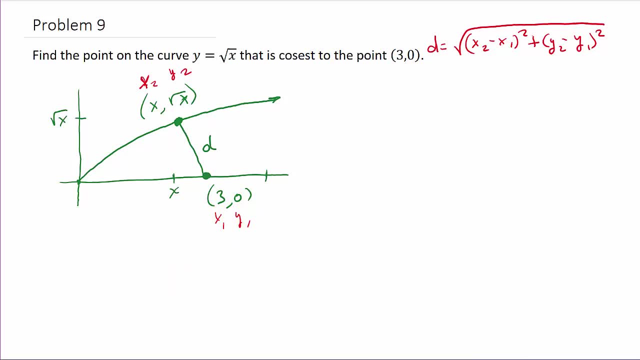 You'll get the same answer, All right. So let's see. Let's see what the distance is. So the distance is the square root of x2 minus x1 squared, plus y2 minus y1 squared. Okay, All right, So the distance is going to be the square root. 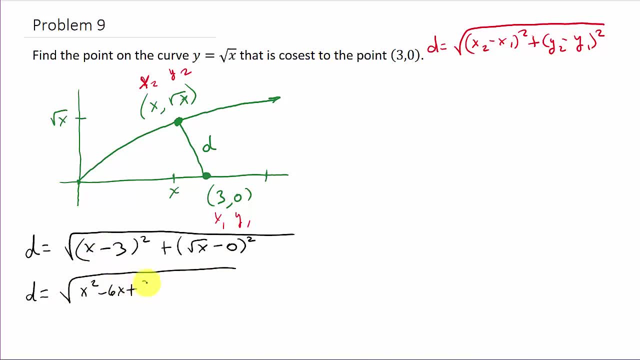 And so this is going to be. So what? x squared minus 6x plus 9 plus? And then this: well, square root of x minus 0 is just square root of x, And then the square root of x squared is x. 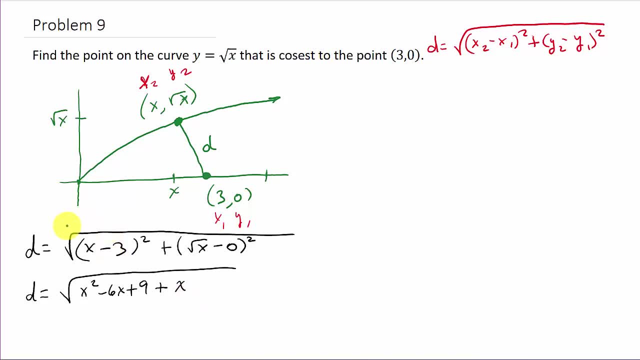 And remember this right here: this x minus 3 squared, just remember that's x minus 3 times x minus 3.. And you fold it out and get the x squared minus 6x plus 9.. And so I get my distance: is x squared minus 5x. 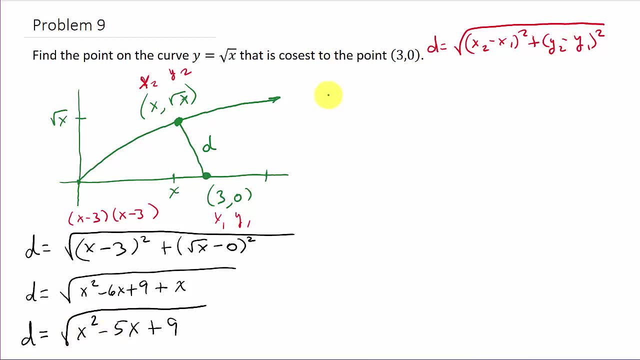 5x plus 9.. So this is my distance. So distance is the square root of x, squared minus 5x plus 9.. That's what we need to minimize, All right, So we've got to take the derivative of this thing. 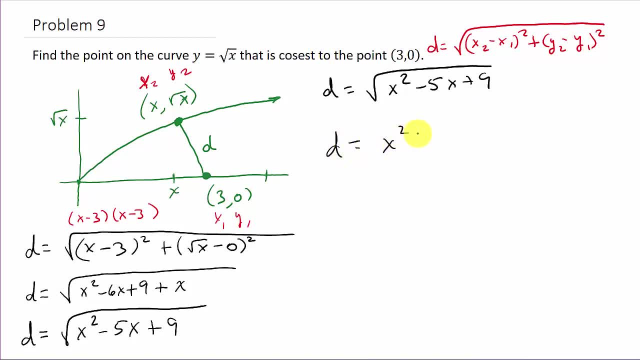 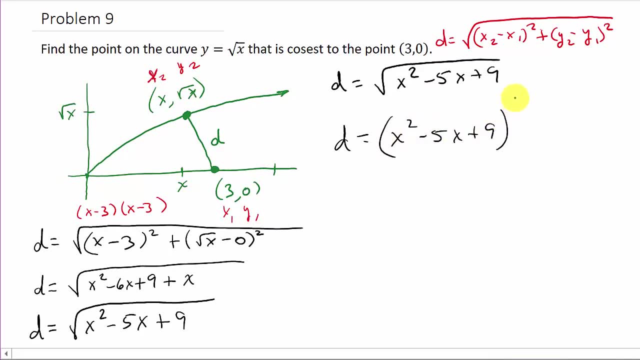 And just real quick, This here: You would change that to an exponent, An exponent of 1 half, And then use the chain rule. Look, there's a shortcut for finding the derivative of a square root. I've got a video on it. 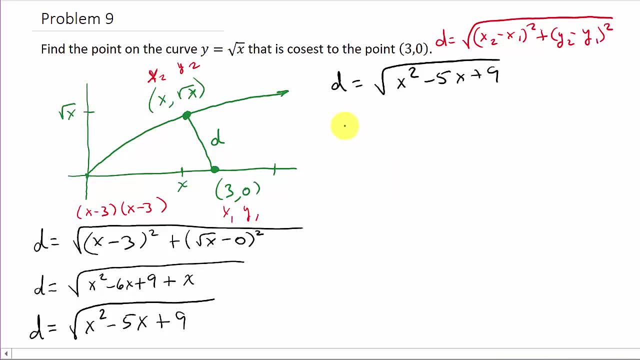 You can search for it on my channel, But I'll show you real quick here. The derivative is Now. to take the derivative of a square root, It's 2 times whatever the square root is. Okay, That goes in the denominator. 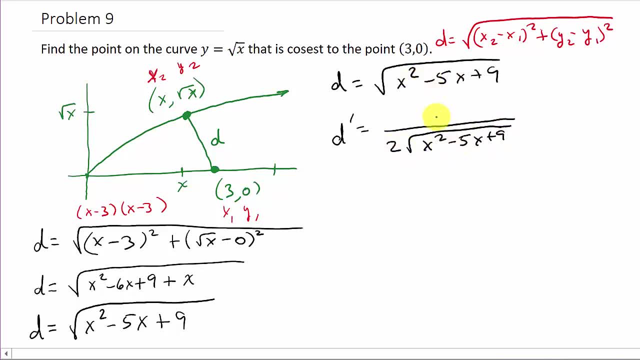 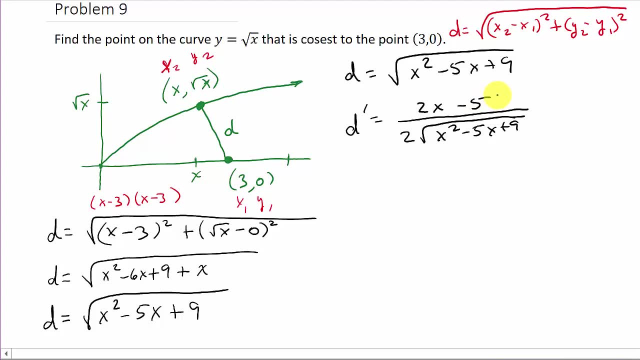 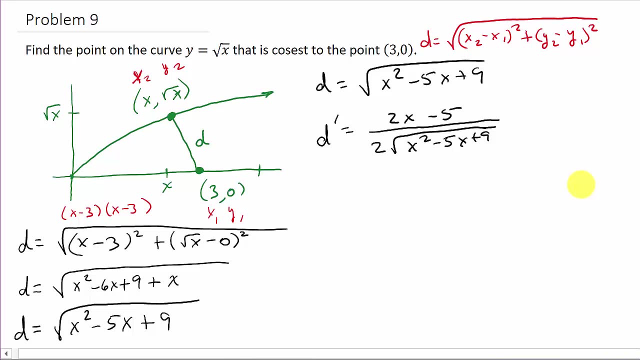 Every time 2 times, whatever this is, And then in the numerator You put the derivative of what's underneath the square root, So that's just 2x minus 5.. Okay, And that's just a quick way to find the derivative of a square root. 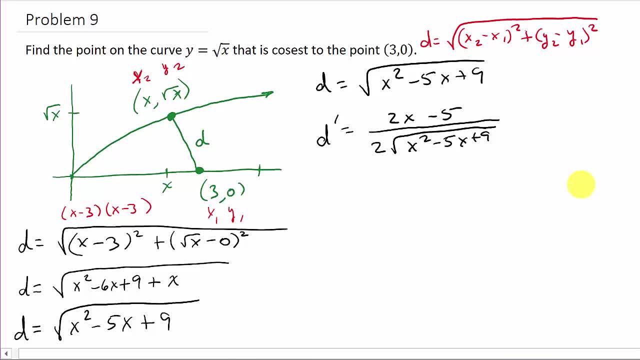 If you want to see more on that, Check the video out. All right, So now we set the derivative equal to 0.. Okay, And solve for x. Well, we know, if we have a fraction, The only time that this is equal to 0.. 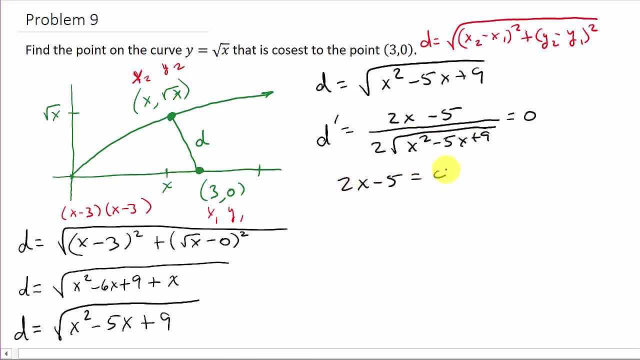 This fraction here Is when the numerator is equal to 0.. And so we set the numerator equal to 0. And so we get x equal 5 halves. All right, Now We have to. Well, we can show that this is a minimum. 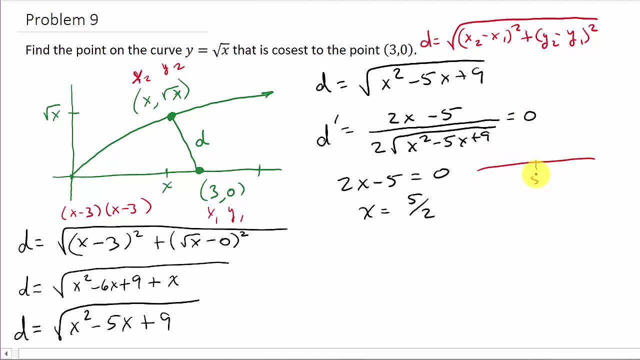 If you, If you draw the line here, Do the 5 halves. Okay, That breaks it up. So this would be what We can use: x equals 0. And we can use x equal 3.. Okay, Well, No. 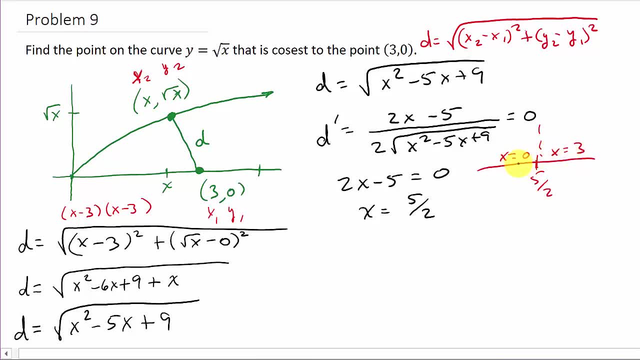 Yeah, We can use 3.. You just need to make sure, Whatever You know, when you pick your x values, Make sure you're in the. You know you're going to have to be in the domain of the radical down here. 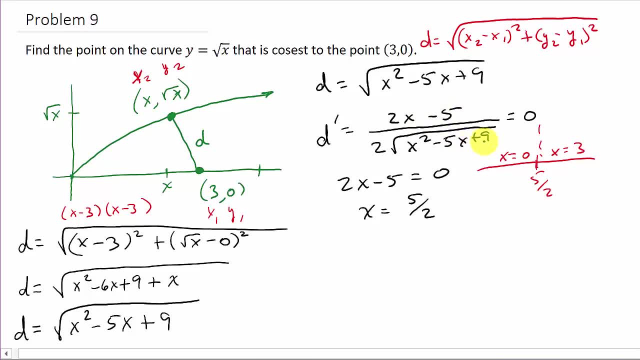 All right. So if we plug the 0 in, Well, when we plug the 0 or the 3 in, The denominator is going to always be positive. And so if we plug the 0 in, We got negative. Negative over a positive is negative. 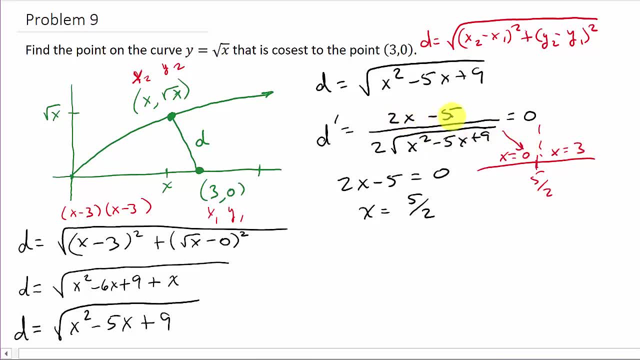 So we can see that's decreasing. Plug the 3 in, That's 6 minus 5.. That's a positive over a positive, That's increasing And you can see we have a minimum There. and so this is our x coordinate: 5 halves. 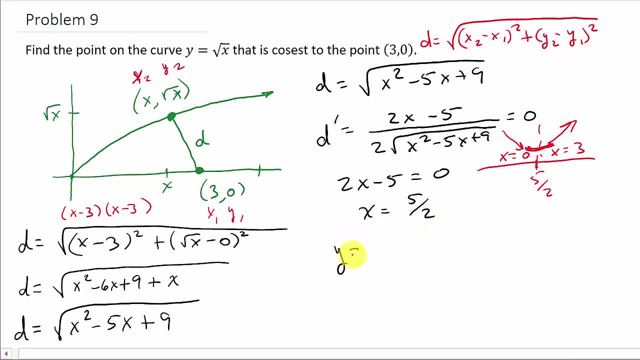 So what's our y coordinate? Well, our y coordinate is: Well, what is y equal? It equals the square root of x, So that's the square root of 5 halves, And so that would give us 5 halves, square root of 5 halves. 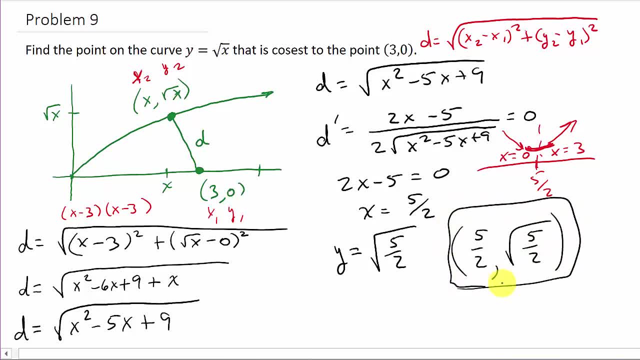 Okay, And this would be your. this would be your solution here. Okay, And you know, if you wanted to, you could rationalize The denominator. you should know how to do that. We would just split that up in the square root of 5 over square root of 2.. 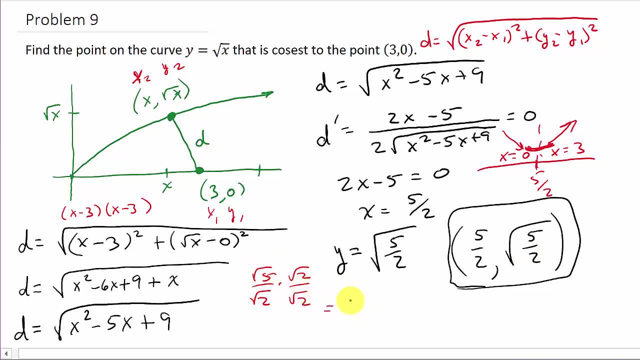 Multiply by square root of 2 over square root of 2.. And that's going to be what: square root of 10 over 2.. So either one, whatever your teacher prefers, All right. So thanks for watching. Give me a like, share and subscribe. Check out my other videos. Thanks,